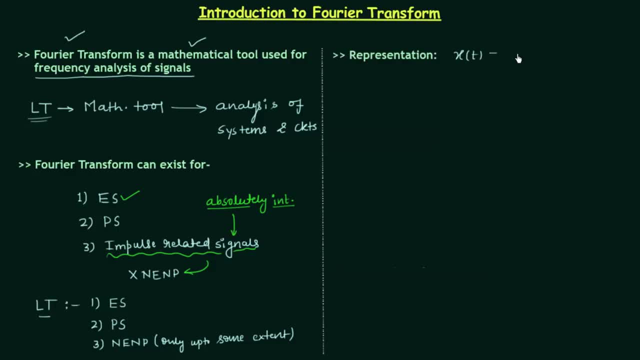 Fourier transform and why we use it. So let's start our discussion by understanding what is. Let's say we have a signal xt, then the Fourier transform of this signal xt is equal to capital X inside the bracket j, omega. There is one more representation, and it is capital X inside the bracket f. 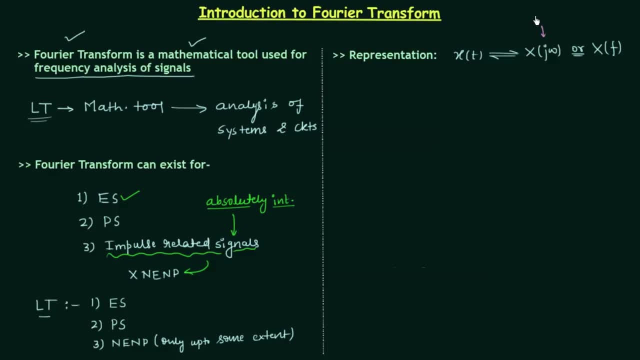 And if we talk about the units, then the first representation is having the unit radians per second and the second representation is having the units hertz And in some books you will find X of j, omega represented as X of omega, and this is to simplify. 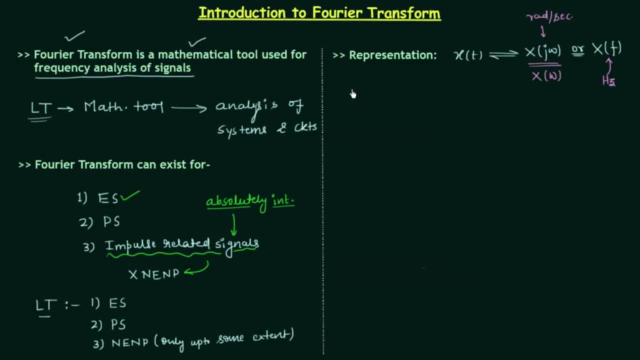 the symbol by omitting j. The Fourier transform of a signal is a complex number. X j omega is a complex number. therefore it will have the magnitude and also the angle. Usually in the questions we are required to calculate X j omega. but if in some question 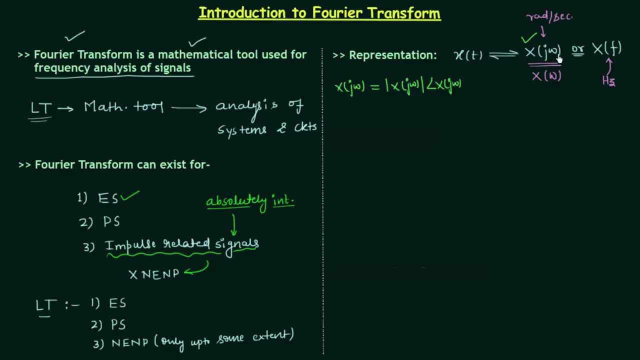 it is asking Xf, Then first calculate X, j, omega and then replace omega by 2pi, f and you will have Xf. So this is all for the representation of Fourier transform, and now we will move to the formulae. The first formula is used to transform the time domain signal xt to the frequency domain. 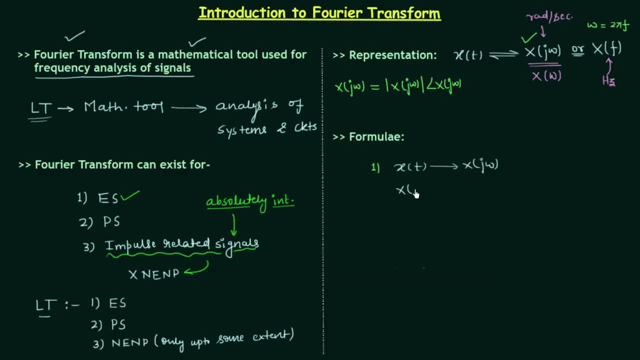 signal X j omega. I will write the formula: X j omega is equal to integration minus integration. The second formula is used to transform the frequency domain signal xt to the time domain signal xt. The third formula is used to transform the time domain signal xt to the frequency domain. 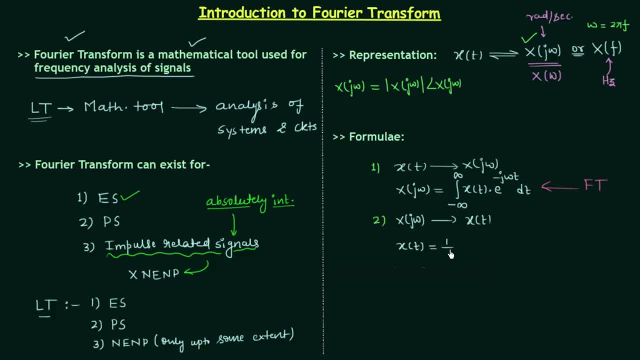 signal xt. The fourth formula is used to transform the time domain signal xt to the frequency domain signal xt to the frequency domain signal xt. The fourth formula is used to transform the time domain signal xt to the frequency domain signal xt to the frequency domain signal xt. 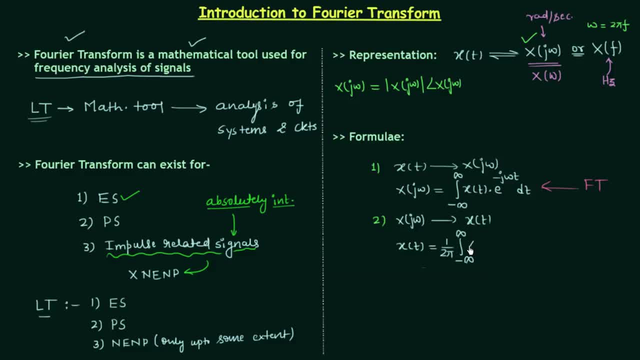 The fifth formula is used to transform the time domain signal xt to the frequency domain signal xt to the frequency domain signal xt. The sixth formula is used to transform the time domain signal xt to the frequency domain signal xt to the frequency domain signal xt. The fifth formula is used to transform the time domain signal xt to the frequency domain signal. 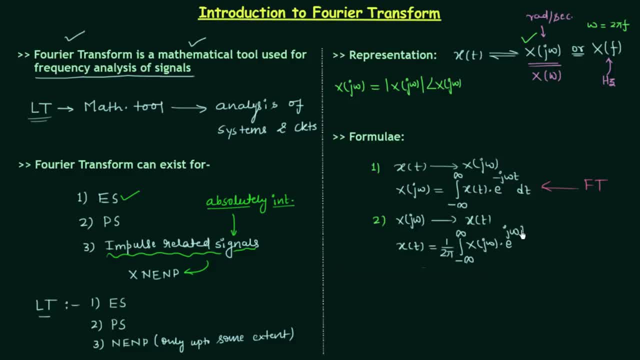 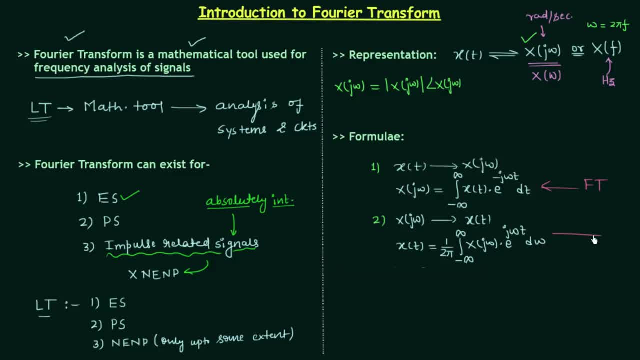 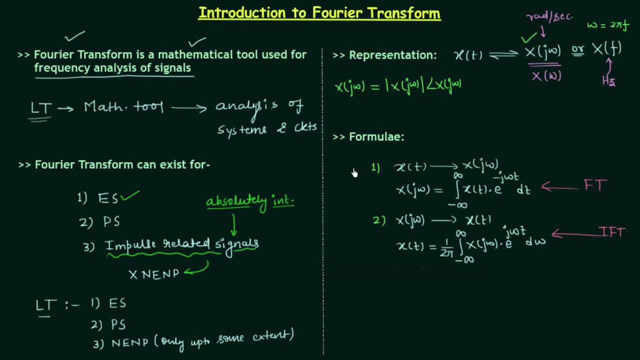 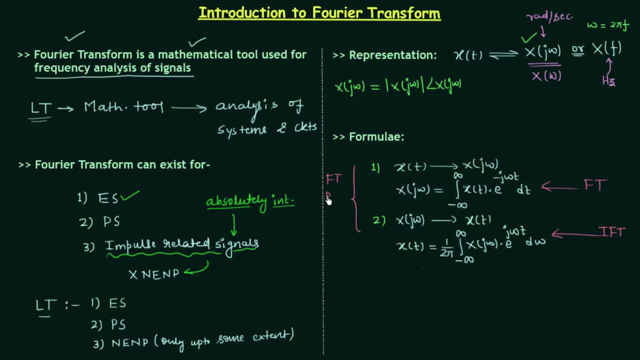 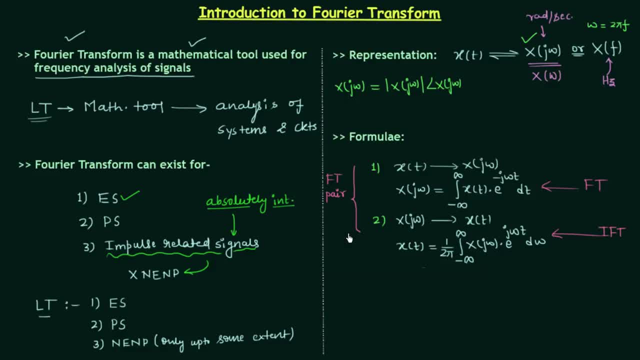 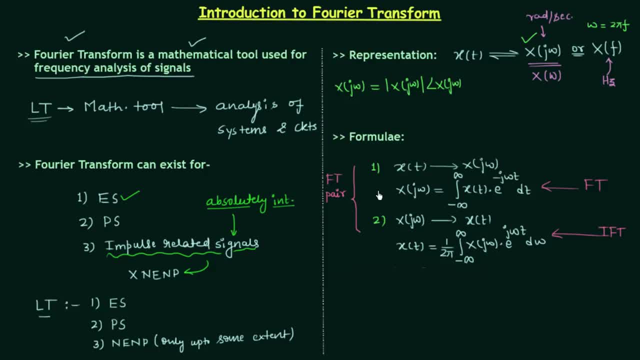 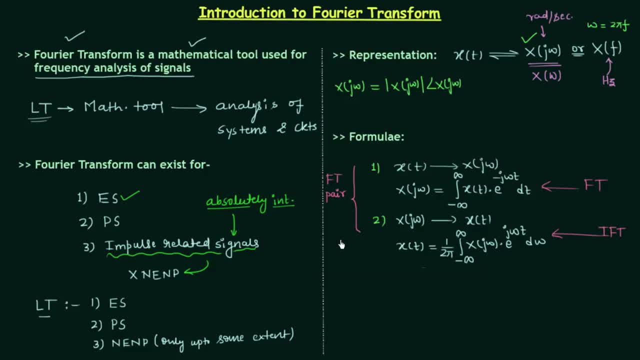 to see this only for absolutely integrable signals, and in the coming presentations we will use the two formulas to solve the questions. Now we will move to the next point, ie The Conversion of Laplace transform to Fourier transform. This point is very important and in the coming presentations I will prove this point. 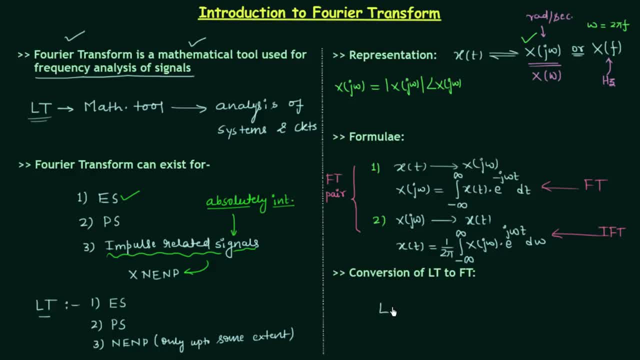 But right now I will just give you the conversion. If you're having the Laplace transform than to get the Fourier transform, simply replace s by, And I will prove this point in a separate lecture. This conversion is valid only for absolutely integrable signals.